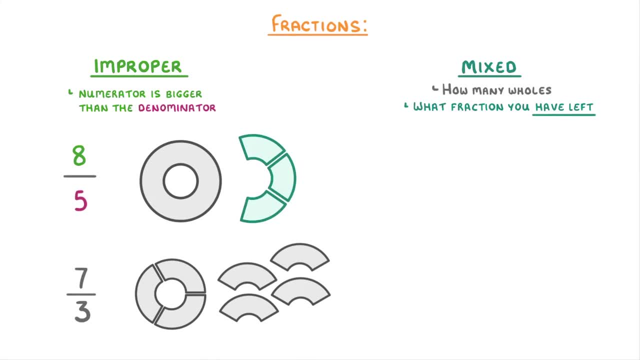 have one whole and three fifths left. So as a mixed number we just write one and three over five. And for our seven thirds, example, we can make two holes and then we have this one third left by itself. So we write it as two and one third. 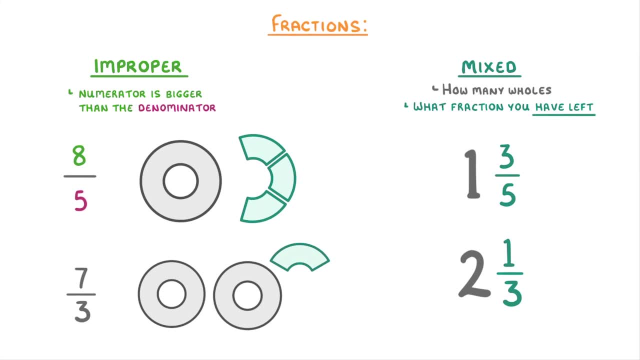 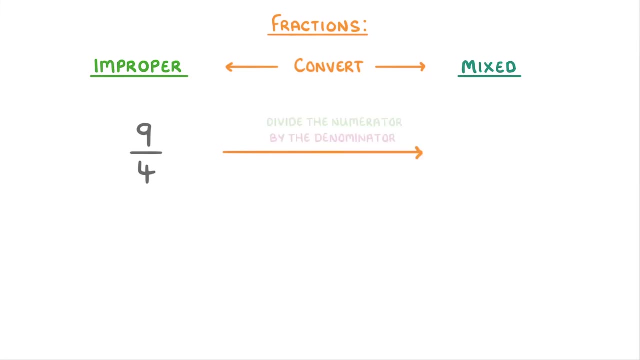 In your exam you could be asked to leave your answer in either form, or sometimes you might have to convert from one form to another. To convert an improper fraction like 9 over 4, into a mixed number, we just divide the numerator. 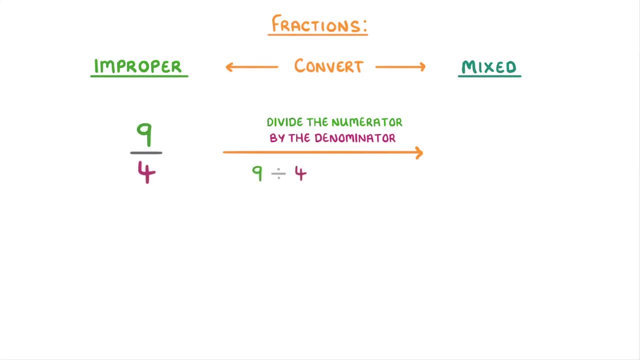 by the denominator, So 9 divided by 4, which is 2 remainder 1.. And so the mixed number form would be two holes and 1 over 4.. Because that remainder of 1 was never actually divided by 4, so it's still a fraction. 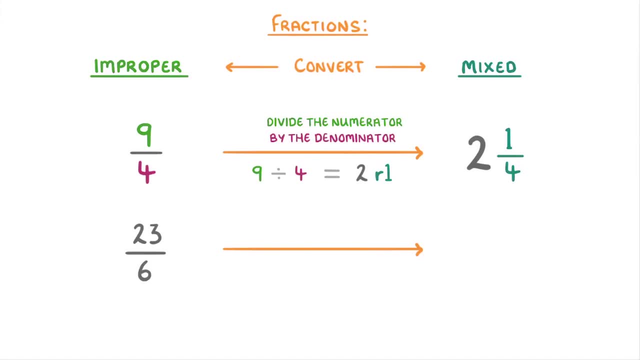 Or if we wanted to convert 23 over 6, we're to just do 23 divided by 6, which is 3 remainder 5.. So the mixed number form would be 3 and 5 sixths. We can also do the opposite and go from a mixed number to an improper fraction. 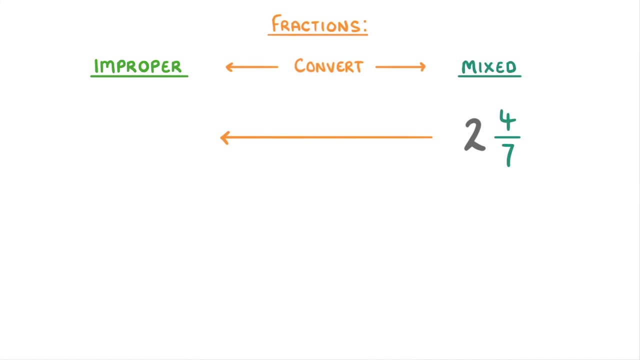 For this we multiply the whole number by the denominator, so 2 times 7, which is 14.. Next we take the 4 sevenths part of the fraction and we add our 14 to the numerator. So our fraction becomes 4 plus 14, all over 7, which we can simplify to 18 over 7.. 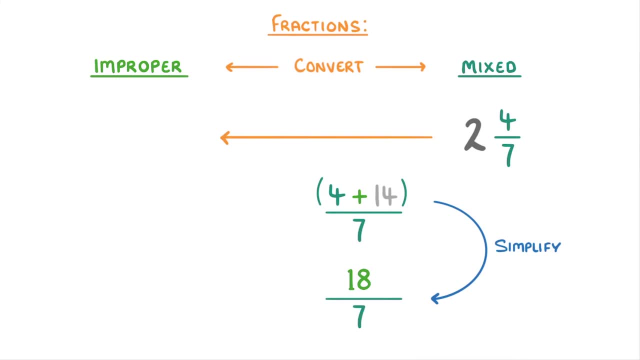 So the improper fraction form of 2 and 4 sevenths is 18 over 7.. Let's try one more. So the first thing we do here is multiply the 3 by the 5 to get 15.. Then we take the 3 fifths. 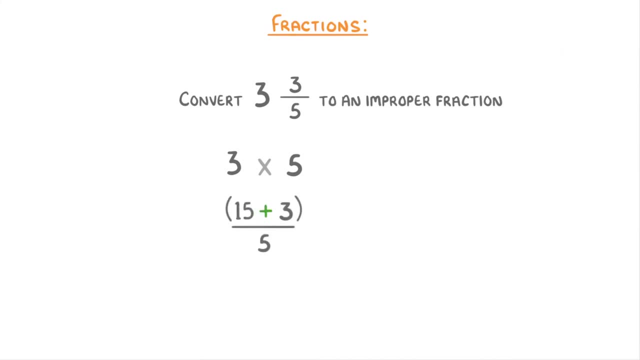 and we add the 15 to the numerator to get 15 plus 3, all over 5, which we just simplify to 18 over 5, which must be our answer, because that is an improper fraction. Anyway, that's everything for this video, so hope you found it helpful.